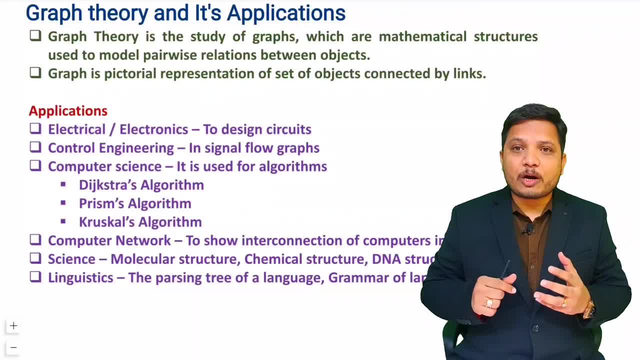 and those graphs are mathematical model of different sets of systems. Those systems may be control systems. those systems may be a circuits which is there regarding electrical or electronics. It may be interconnection of computers. There are many applications which is there, along with graph theories. So graph theory that explains graphical representation. 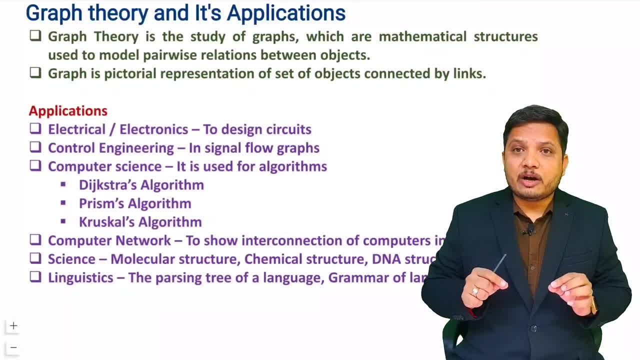 or you can say pictorial representation of any system in which, whatever nature is there with different objects. That may not be covered, but it shows how connection is there and how it will be reacting to the different sets of inputs, So different elements and all those things that I'll be explaining. 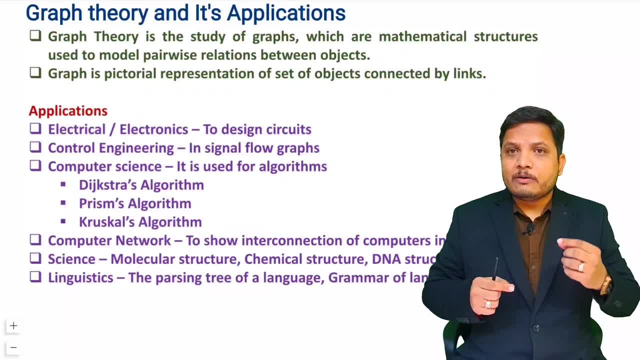 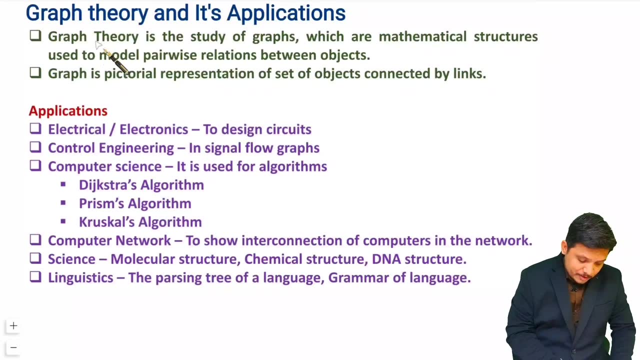 you in next videos. In this video, what we will be doing is I'll be explaining you basic meaning of graph theory and what are the applications which is there with graph theory. So, as I said, graph theory is a study of graphs, which are mathematical structure used to model pairwise. 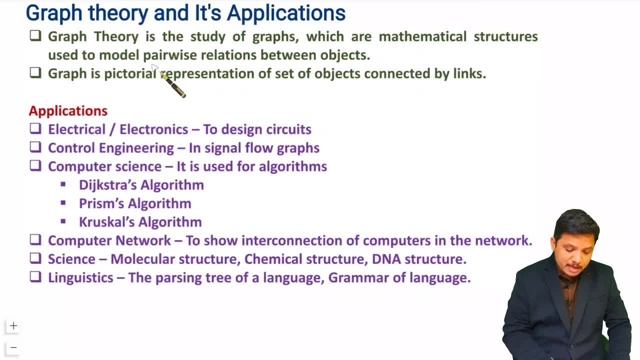 relation between objects. So here objects may be related control system. It may be there in terms of circuit, It may be there in terms of connection in between computers, So that we will discuss in application part. See graph is a pictorial representation of sets of object connected by. 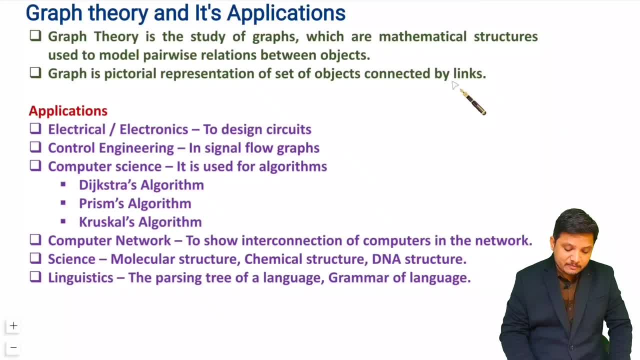 links. So we will see Different types of graph in next further videos. Let us discuss what are the applications which is there with graph theories. So when we talk about applications in electrical and electronics we use graph theory to design the circuits. So in this playlist of network theory I'll 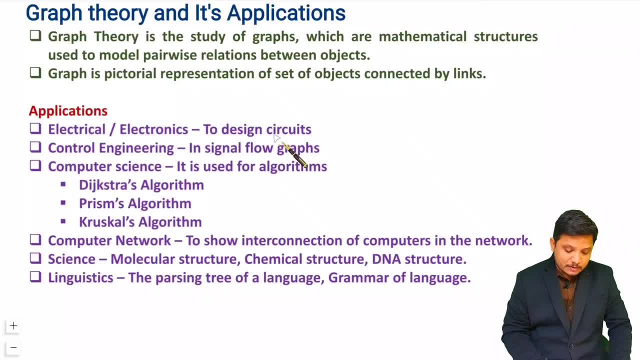 explain you how we can design the circuits using graph theory. You will be observing in control engineering using signal flow graph. We use graph theory, So signal flow graph. those are used to identify transfer function of the system in which we observe how connection is there in between nodes and how final transfer. 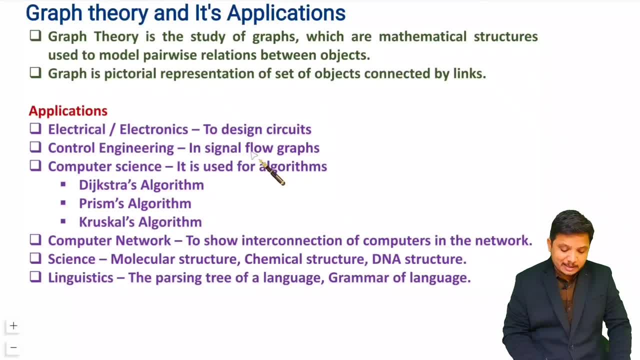 function is there of whatever system that is connected in graph. So that is what the part which I have already covered in control engineering- You will be observing. in computer science It is used for algorithms like Dijakastra algorithm, Prism algorithm, Krushkal algorithm. So those algorithms, 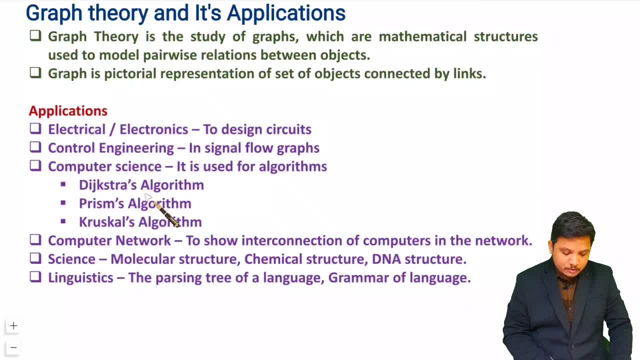 are there in which graph theory is being used. These algorithms are used to find shortest path from transmitter to receiver. These algorithms are also used to identify maximum bandwidth path or you can say possible paths in between transmitter and receiver. So there are many other applications which is there with graph theory in computer science, but here I have. 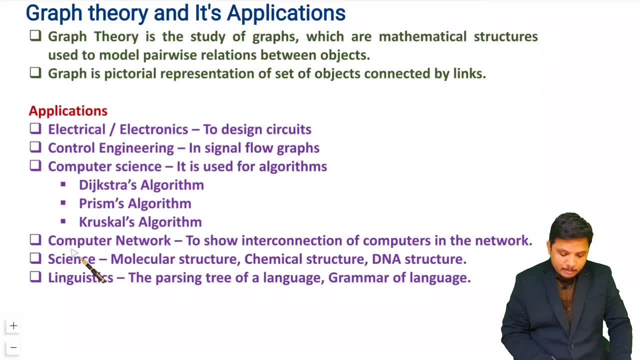 listed these algorithms only When we talk about computer network. so it is used to show interconnection in between computers in the network. and you will be observing, in network simulator we use graph theory in which computers are connected in between each other and whatever bandwidth is associated with computer or whatever data rate is being provided in between computer. 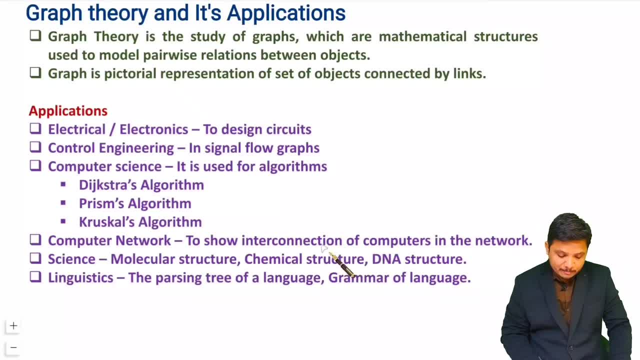 all those things that we can simulate in network simulator. So in computer network also there is very essential application, which is to identify computer network along with the speed connected in between two nodes, as well, as it is also used to identify possible path, as well as it is also 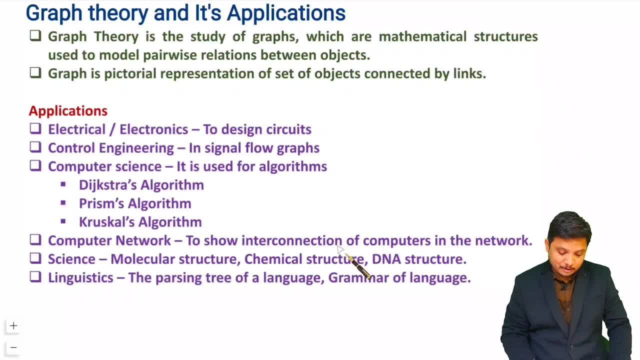 used to identify how we can correct and detect error In science. there are many applications. I have listed few only like molecular structure, chemical structure that can be studied, chemical structure that we can study by using graph theory, as well as DNA structure that can be established by using graph theory. You will 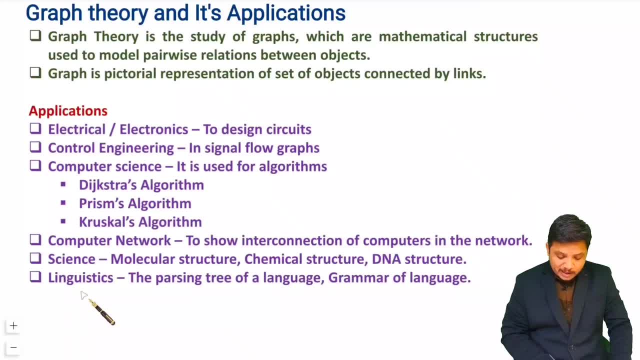 be surprised to know that in linguistics we use graph theory, in which the parsing tree of language can be studied by using graph theory as well as grammar of the language that is also based on graph theory. So whenever you form any statement at a time in sequence, 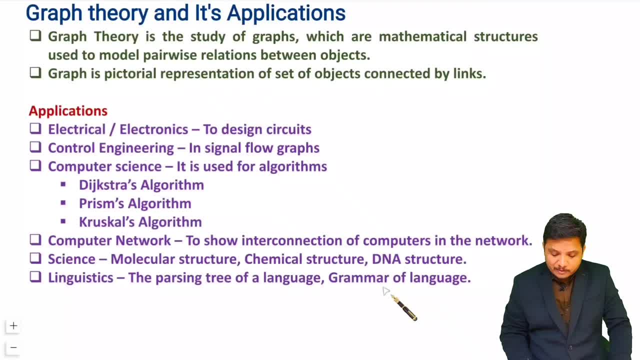 it should follow some trees. If it is not following well-defined trees, in that case computer automatically identifies that there is grammatical error In word file. you might be observing that if green line is coming below your statement, in that case it shows.